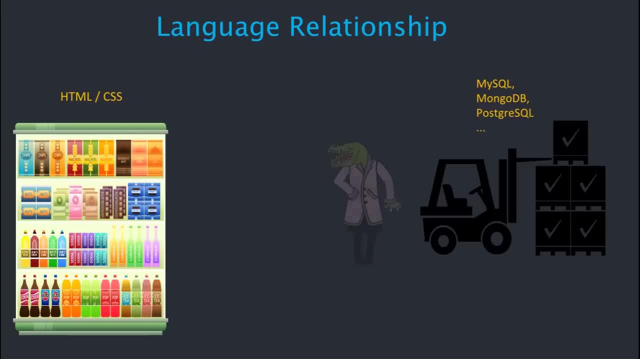 even slow down your entire application. Standing right in front of our database, we have Alligator Server-Side Code Woman. She's kind of like the store manager. She can communicate with the warehouse workers, also known as the database management system. She can also perform calculations, manipulations and had. 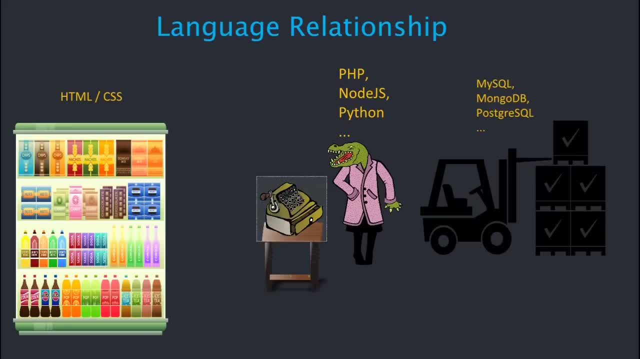 security clearance to deal with sensitive information. She's often in charge of the application's logic and infrastructure. However, she isn't the best at dealing with customers, So at the front of the store we have our customer service manager, JavaScript. JavaScript works on the client side. It can interact. 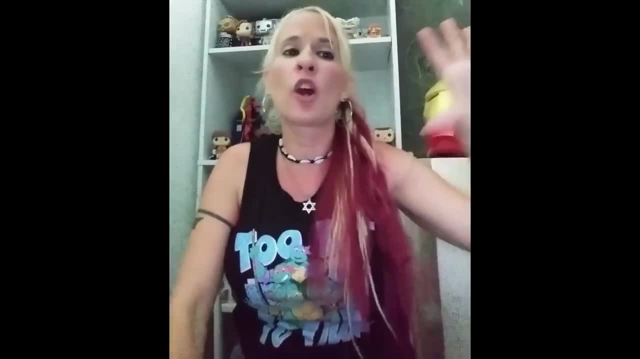 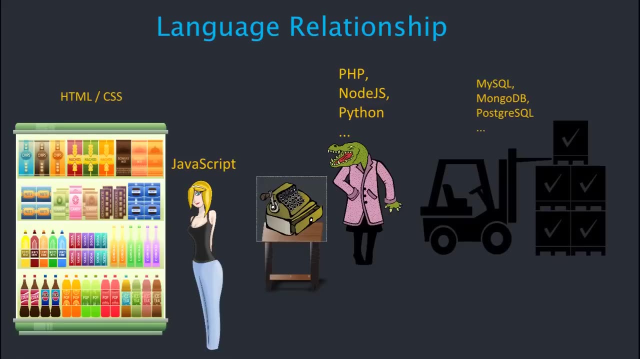 with the HTML and CSS, It can go in the front of the house and talk to the designers and the clients to make sure our display shelves are displayed in a user-friendly manner. She can also perform calculations and manipulations on non-secured data that is passed to her from Alligator Sericide Code Woman. 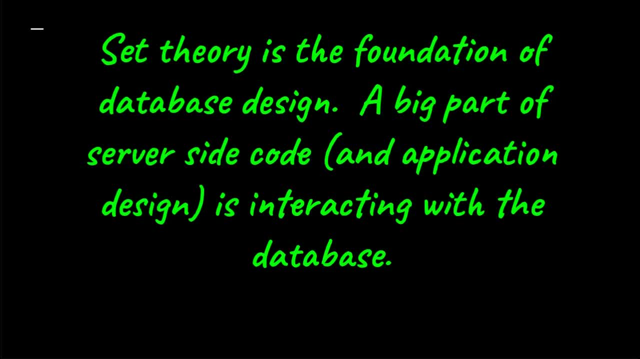 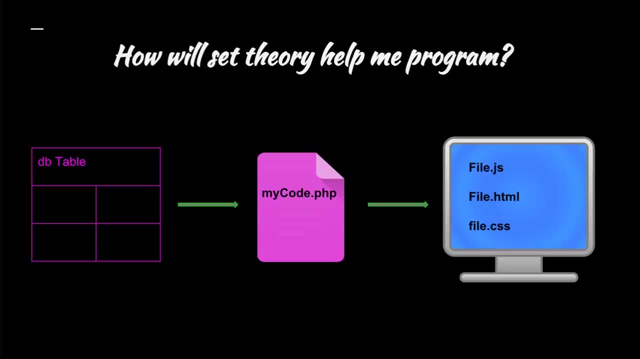 Set theory is the foundation of database design. A big part of Sericide Code and application design is interacting with the database. So if you become a logic rock star, it's going to be a whole lot easier for you to design solid applications. As a matter of fact, in computer programming we have data types. 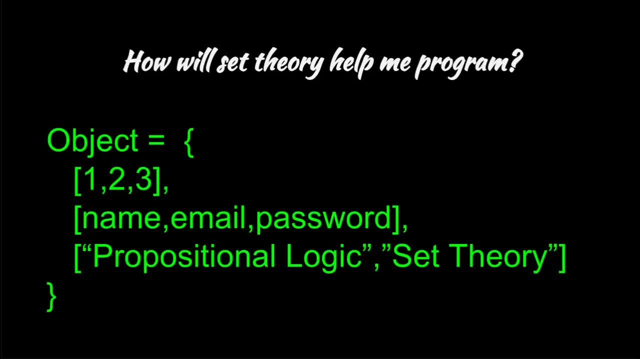 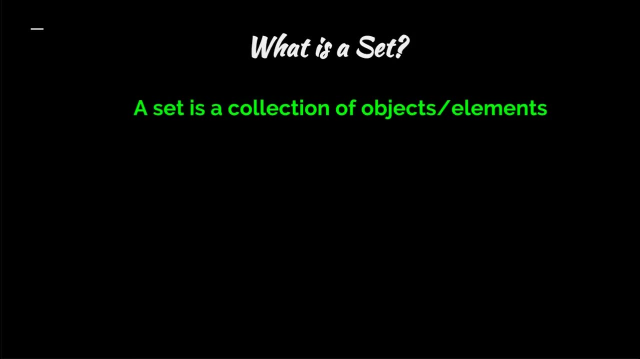 called arrays and objects. These data types are used for storing sets of data. These data sets are often directly defined by our database tables. So next you might be wondering: what is a set? A set is a collection of objects or elements, Say. 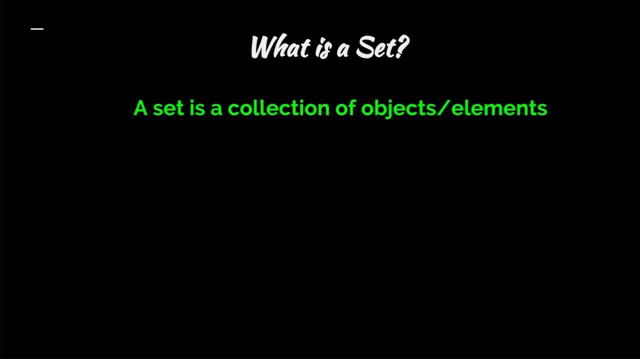 you're designing a login page, You'll deal with sets of user data. Each user object may be a set of data including username, email and password. You may also be dealing with a set of user objects. In mathematics we say x is an. 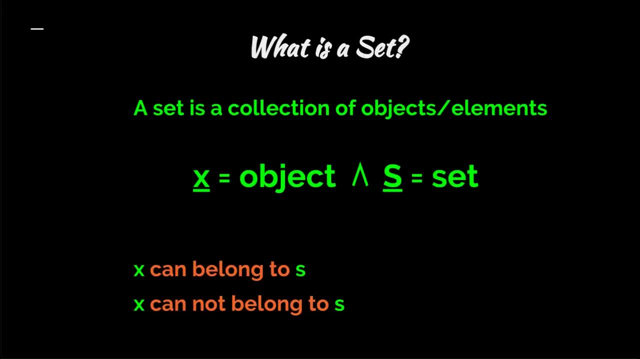 object and s is a set. If the above statement is true, then x can either belong to s or x cannot belong to s. If you remember back to my intro to propositional logic video, a proposition is a statement that can either be true. 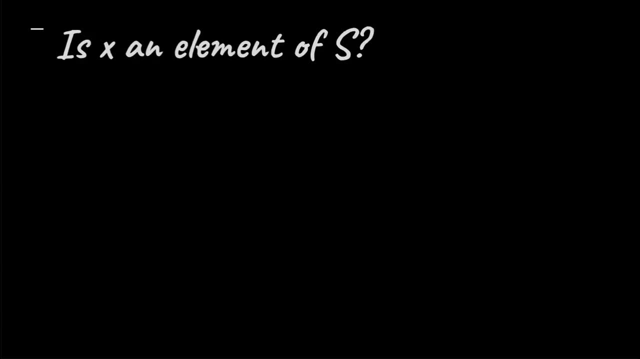 or false. The statement x is an element of s can be true, x or false. It can be true or it can be false, but it can't be both In mathematics. if it's true, we say x is an element of s and is denoted just like. 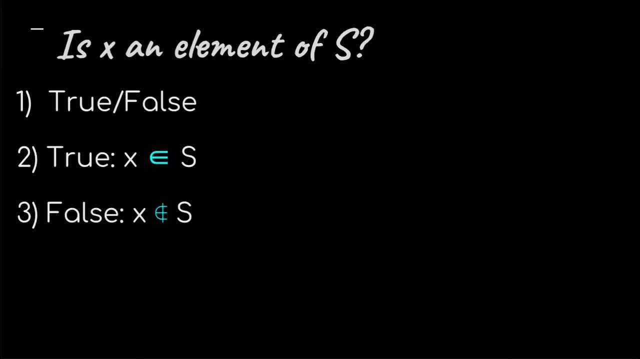 you see, And if x is not a member of s, we denote it like this. Let's say, set s is equal to all possible even numbers. You tell me, are the following statements true or false? 2 is an S. Yes, that is true. 2 is an even number. 3 is an element of S. Nope, 3 is odd, It's. 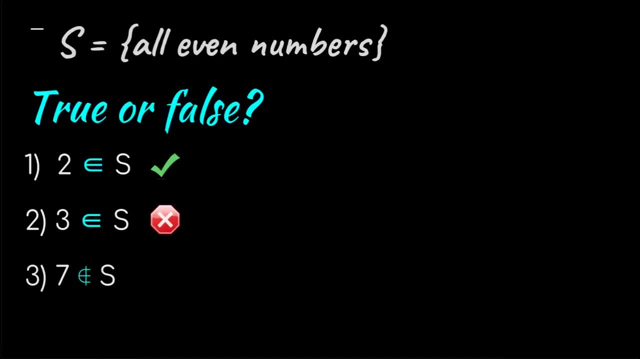 not even 7 is not an element of S. That's true. 7 is not an element of S because 7 is odd. How do you define a set? There's two ways to define a set. The first way is by: 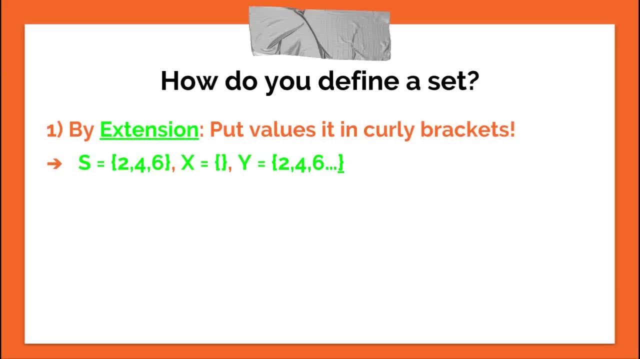 extension, And we do that like so by putting values into curly brackets. We have S equals 2,, 4,, 6.. And then we have X equals an empty set- There's no values in there- And Y equals basically all even numbers starting at 2.. What that dot dot dot means is that the 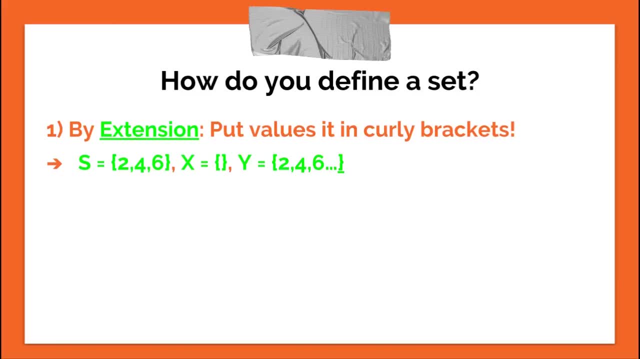 pattern is going to continue, So Y is going to equal 2,, 4,, 6,, 8,, 10,, 12, and so on. The second way we can define a set is by intention, That's definition by membership. 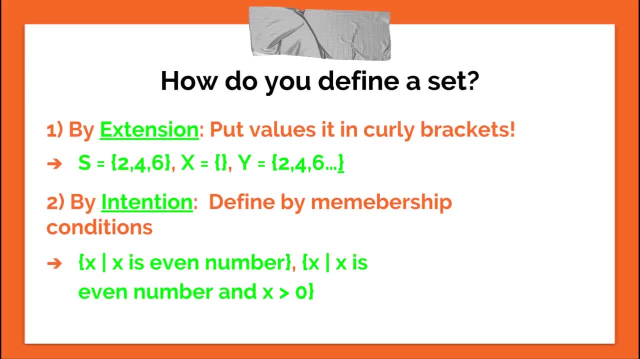 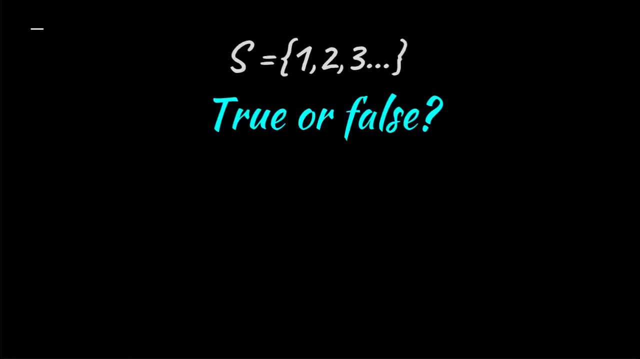 condition. So we could say X is a member if X is an even number. Or in the second example, X is a member such that X is an even number and it's also greater than 0. S is going to equal the set of all real counting numbers. Tell me, are these statements true or false? 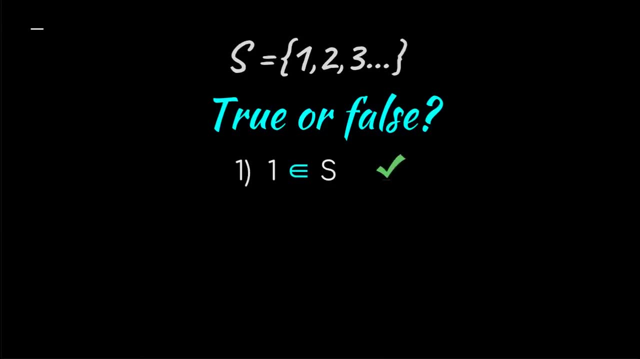 1 is an element of S. True 1,000 is an element of S. 1,000 is a real counting number. That is true. Negative 1,000 is not an element of S. That is true as well. X, such that X. 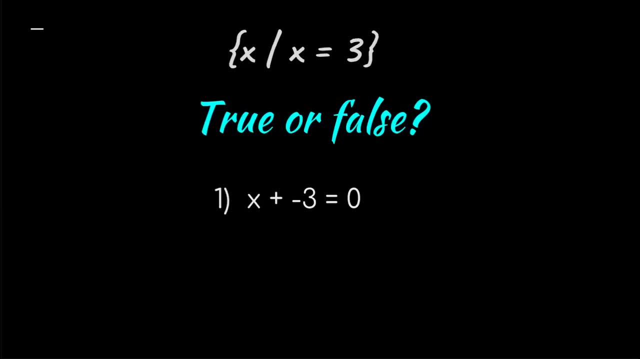 equals 3.. X plus negative 3 equals 0. True, because 3 plus negative 3 equals 0.. X is less than 0. Err, false: If X equals 3, then X must be greater than 0. So this: 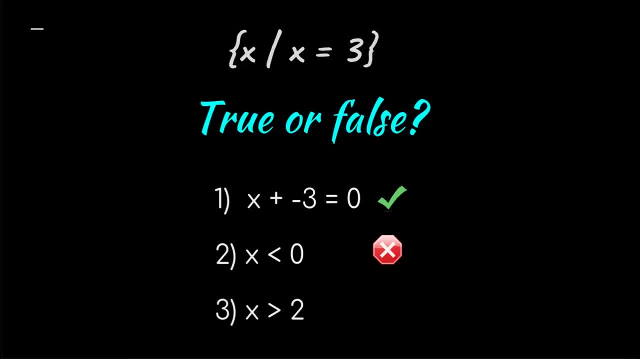 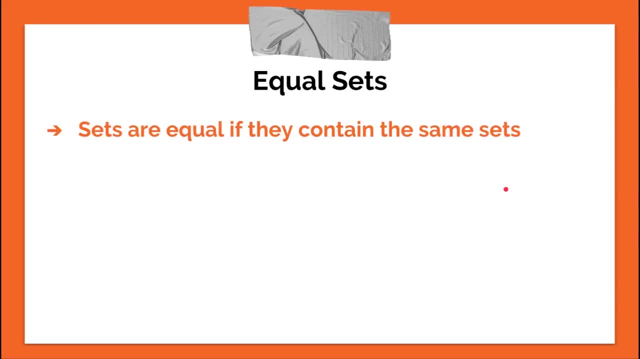 is false. X is greater than 2.. True, because 3,- yes indeed- is greater than 2.. Sets are equal if they contain the exact same elements, and order doesn't matter. So if S equals 1,, 2, and 3.. 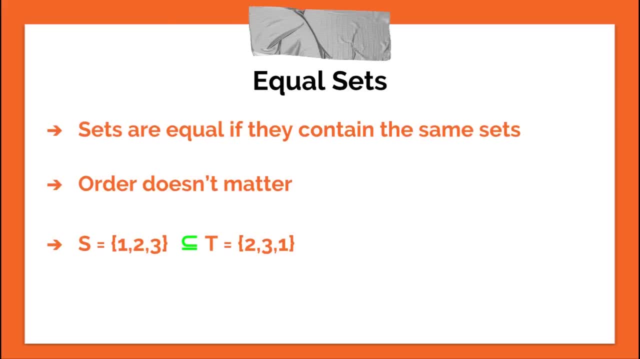 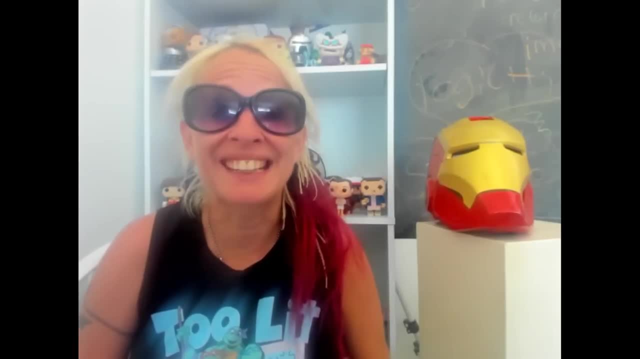 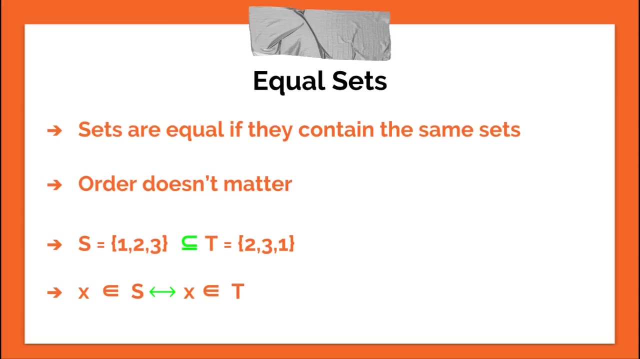 And T equals 2,, 3, and 1.. S and T are still equal sets. And if sets are equal, remember by conditionals from intro to propositional logic, X is an element of S. if, and only if, X is an element of T subsets. If all of A's elements are contained in B, then we say A. 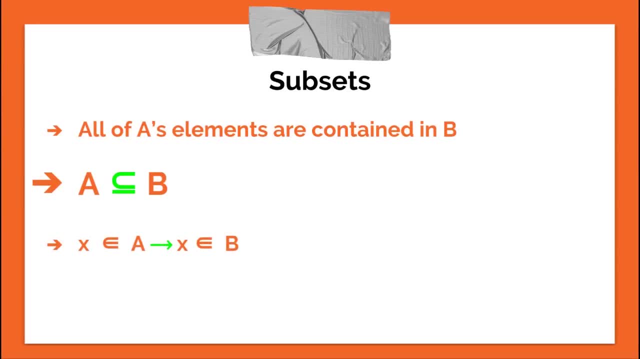 is a subset of B. So if A is a subset of B and X is an element contained in A, then X has to also be an element contained in B. Null set. That means it's completely empty. There's no values in it. 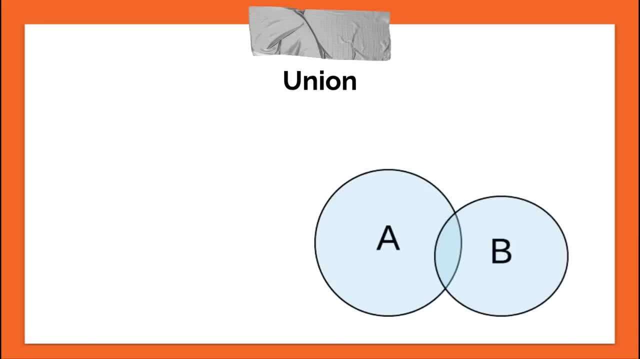 And we write it like that: Union. OK, Look at that diagram with A and B, A union B, X, such that X is an element of A or X is an element of B. If you look in the diagram, everything in A and everything in B is going to be included in A union B. 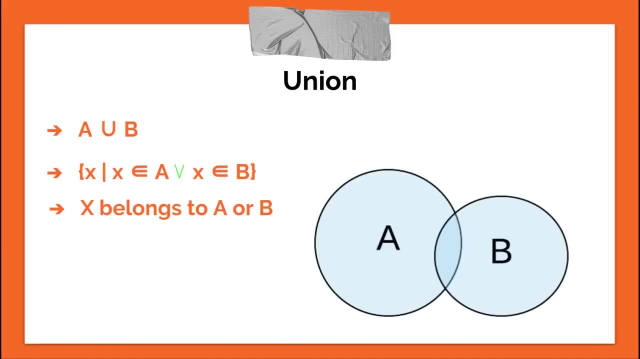 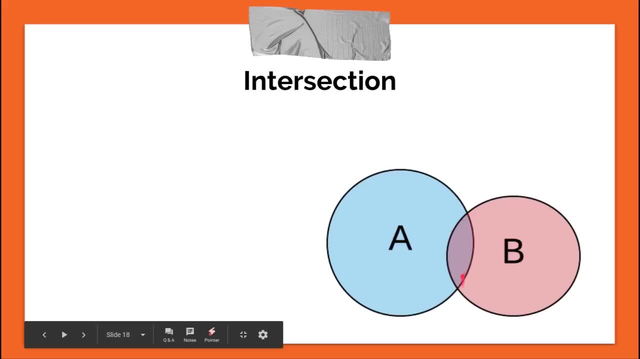 X belongs to A or it could belong to B. Either one Intersection. Intersection is going to be this area. I tried to make it kind of purple, combining the blue and the pink X such that X is an element of A and X is an element of B. 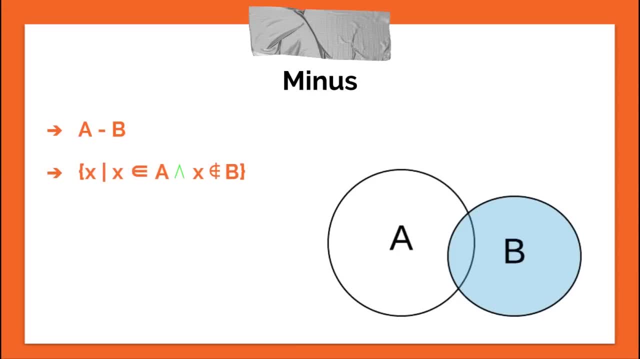 A minus B- X, such that X is an element of A and X is not an element of B. Okay, So if you look here, this white area that's not shaded, that would be A minus B. The elements contain an A. 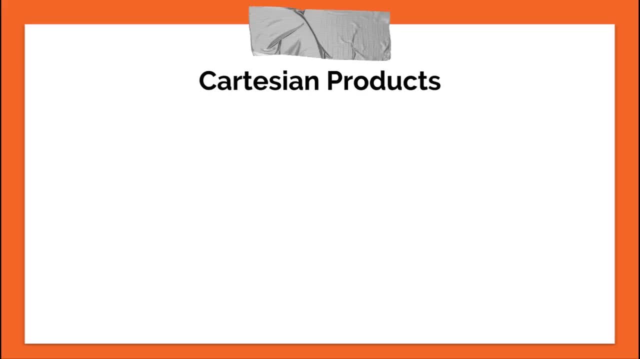 That's A and B Cartesian products. Okay, Just relax for a second and sit back and just get the concept. The Cartesian product is the product of two sets. Say A is a set which contains the values A, B and C, and B is a set that contains the values X and Y. 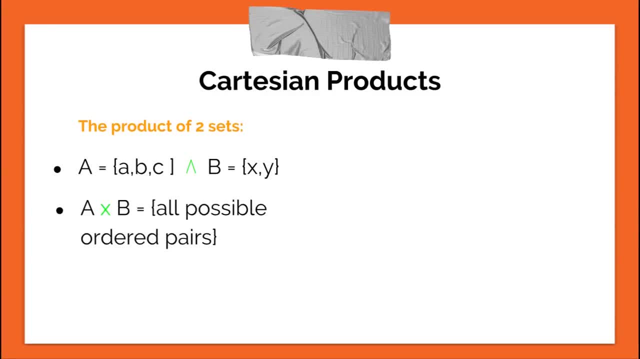 We would write the Cartesian product as A times B. Now, if we put the value in the correct order, we would have an A times B. If we take the A, we would have an A and then we would have an A. Okay, so what are the proper ordering pairs? 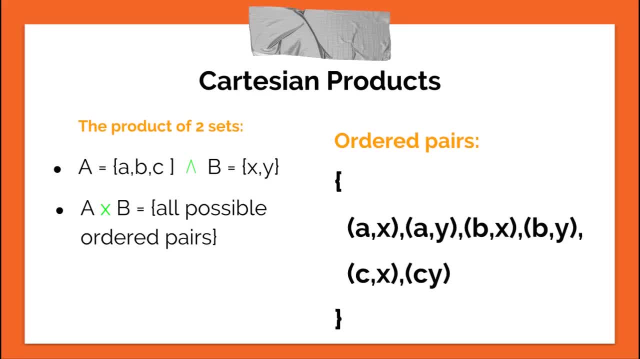 We have the manual, we have the x-axis, we have the y-axis, we have the y-axis, we have the y-axis and we have the z-axis, the y-axis and the y-axis. Now, what is the proper ordering pair for this? So we have to do some math here. What is the proper ordering pair? All possible ordered pairs can equal all possible ordered pairs. Ordered pairs are when we take an element in A and we match it with an element in B. So all possible ordered pairs are going to be AX, AY, BX, BY CX and CY. 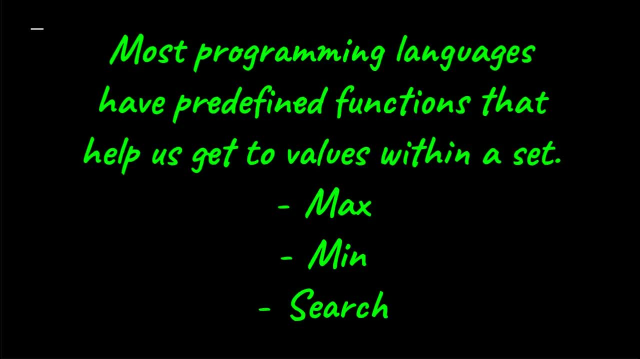 Most programming languages also have a common order, and that is x and C have some predefined functions that are going to help us find values within a set. Because of that, I'm going to spare you all the mathematical equations to calculate these things. Most of 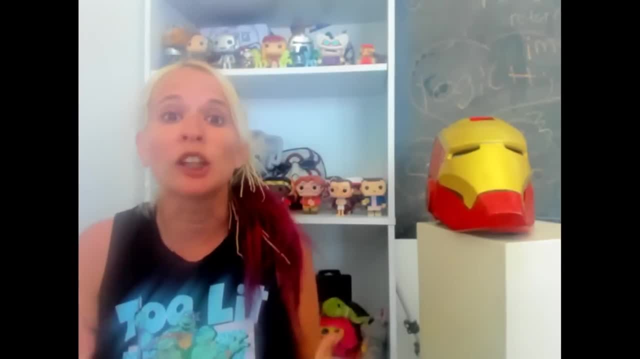 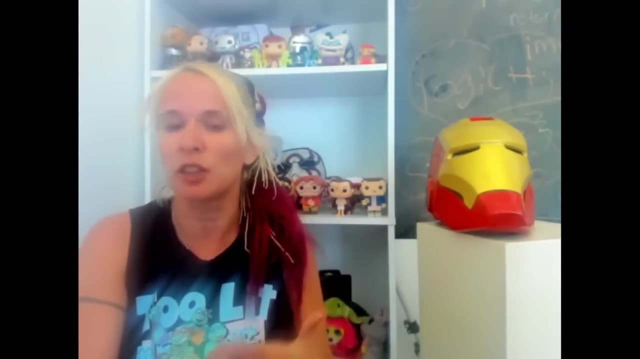 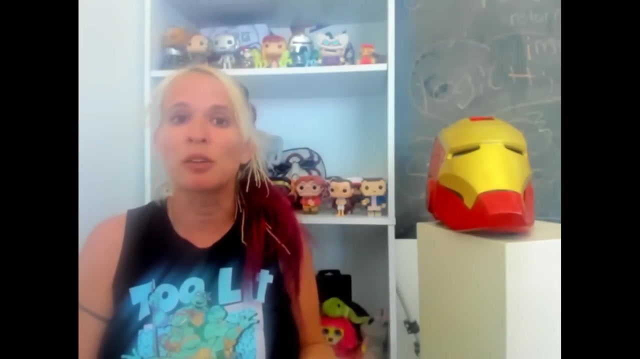 them. I think we know what they mean. Like we might have a set of values and we want to find out what's the biggest value in there. that would be finding the max value of the set. Most programming languages have a function for that. If we want to find the smallest value in a set, we'll look for the. 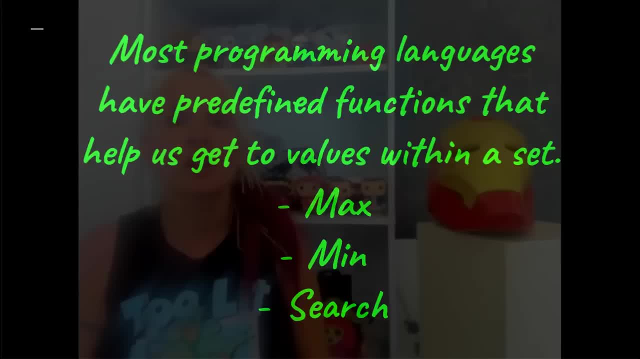 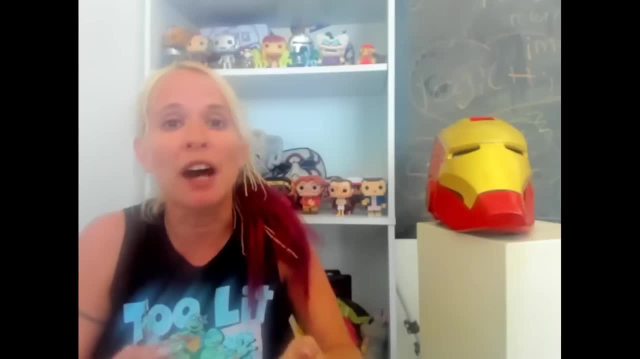 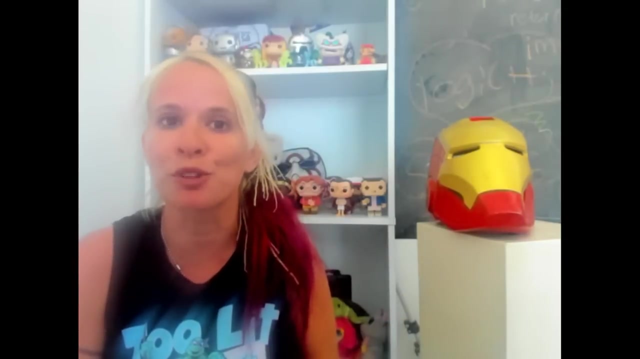 minimum, Most programming languages have a function for that. For a search. we could want to search for all kinds of things And programming languages do tend to have different predefined functions where you might be searching for a particular string. Say you want to return any members of? 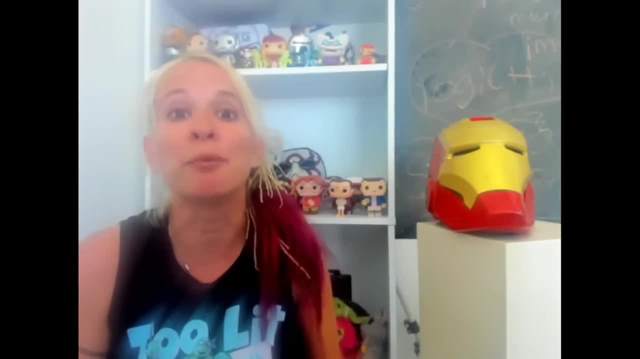 the set that contain IMG. You're looking for image content. Or maybe you're looking for a set of images that contain IMG. Or maybe you're looking for a set of images that contain IMG. Or maybe you're looking for a set of images that contain IMG, Or maybe you're looking 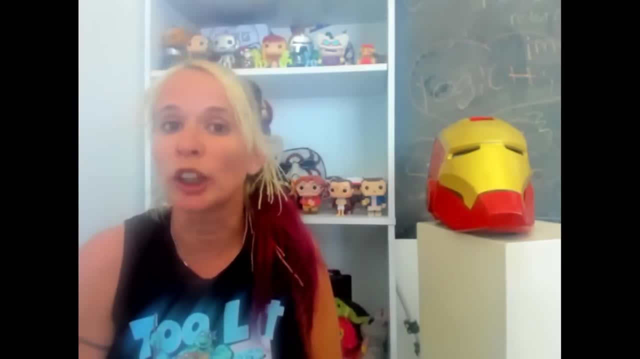 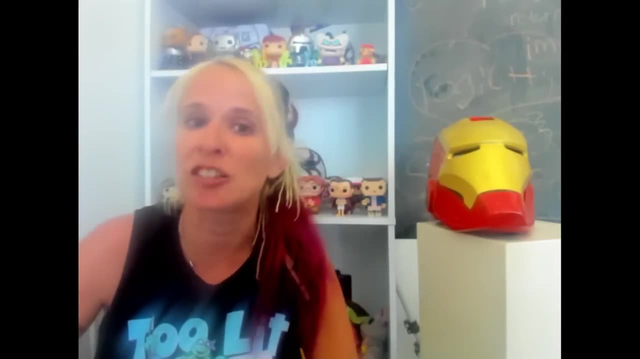 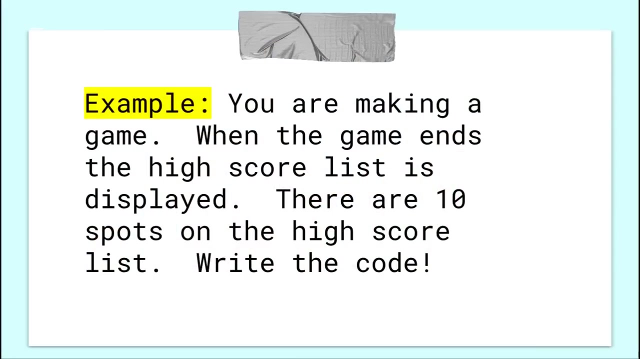 for a specific value. Maybe you are looking for the blog article that was posted on a specific date, So you're searching through the dates for the one that matches. Most programming languages have predefined functions to handle all this kind of stuff, So let's do an example, Okay. 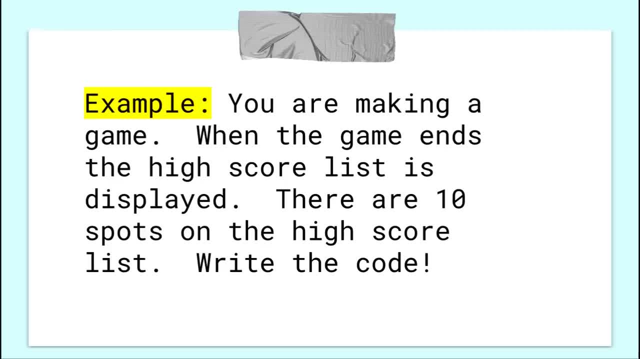 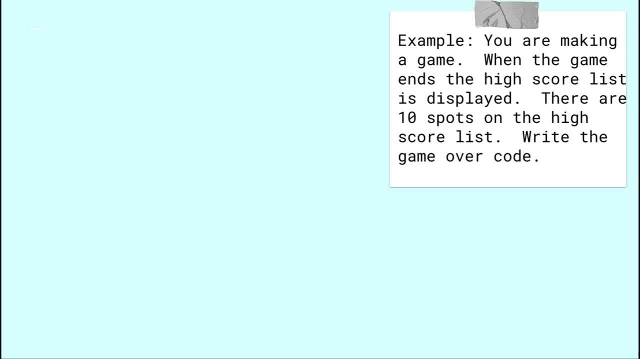 you're making a game. When the game ends, the high score list is displayed. There are 10 spots on the high score list. Write the code: Okay. so, for example, let's do the logic thing. Let's let t equal total score, h equals high scores and s equals show high scores. 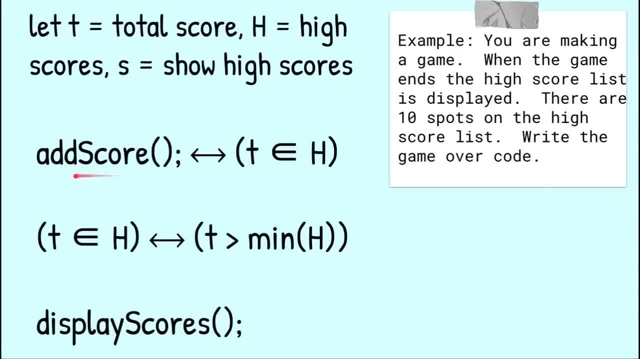 Just in case the total score qualifies, we're gonna have a function written somewhere to add that score to the high score list. We want the code addScore to execute if, and only if, total score is an element of the high score. So if we have a high score and the total score is a function, we want that number of values to add a value to the high score. 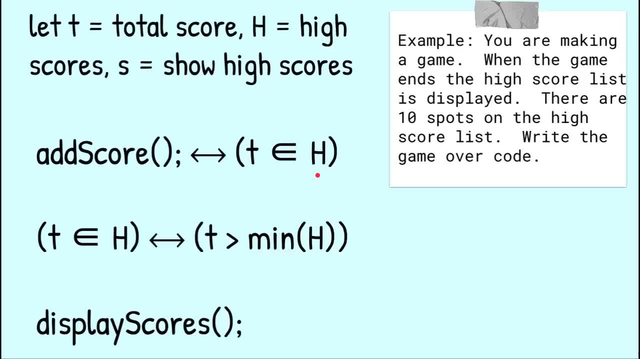 of all the values you can add to the high score. we want that number of values to add a value to the high score on the high score list and total score is going to be included as a member on the high score list if, and only if, the total score is greater than the minimum. 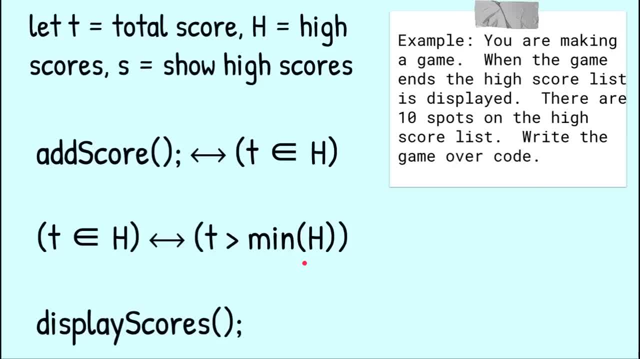 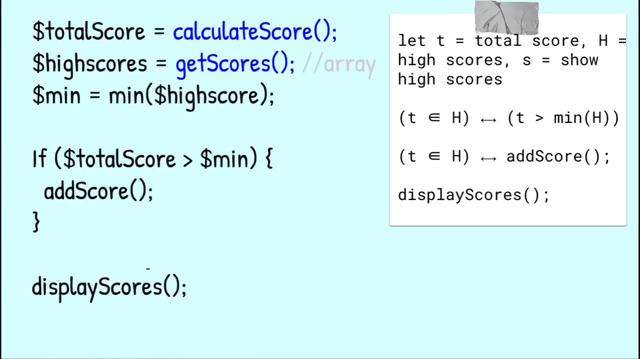 score on the high score list, the smallest value there and regardless. we are going to display the high score list somewhere. we're gonna have a function with code to display the top 10 scores and if your total score qualifies, you will see your name and score there. so let's write it in PHP. we have dollar sign. 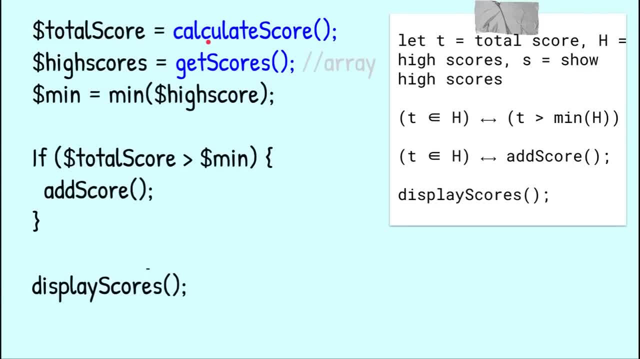 total score equal to a function that we have written out elsewhere which calculates the current players. total score. dollar sign- high scores is going to equal another function that we have someplace else which is probably have a query there to go ahead. go to the database, get those 10. 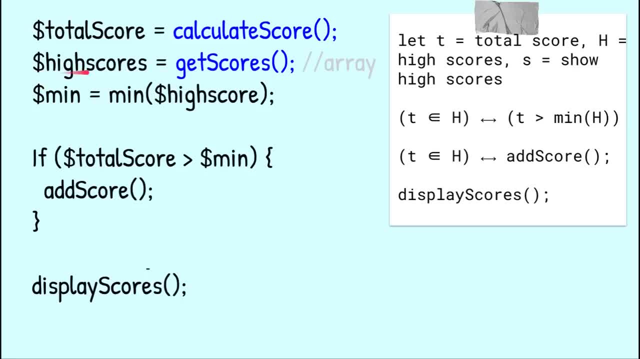 high scores and we'll store it in dollar sign high scores. dollar sign min. in PHP we do have a predefined function to find the minimum value in a set, so dollar sign min is going to equal the minimum of dollar sign high scores if total score is greater than the minimum. 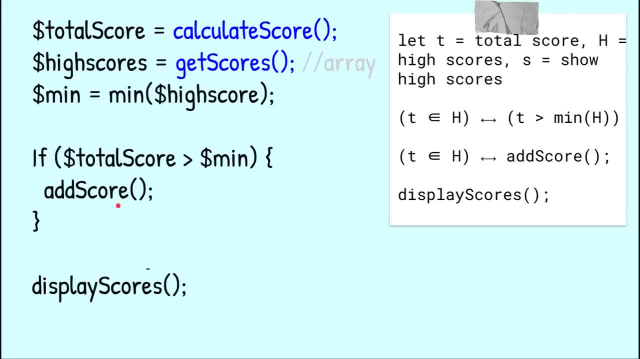 then we're going to execute the code to add the total score to the high score list and no matter what. in any case, we will display the high score list for everybody to see. if you made it as a member on the high score list, you will see your name there. if you did not, you will still see the chosen ones who did. 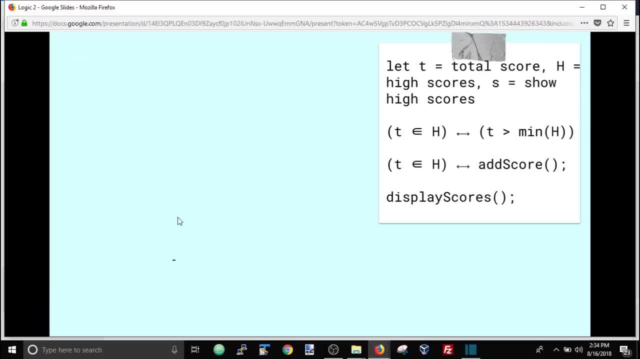 make it on the high score list. now let's check it out. in JavaScript, we have three он High scores equaling that function to calculate the current total score. we have our high scores equaling that function. to go the database and get the high scores, we have var min equaling. and JavaScript, we also have a predefined 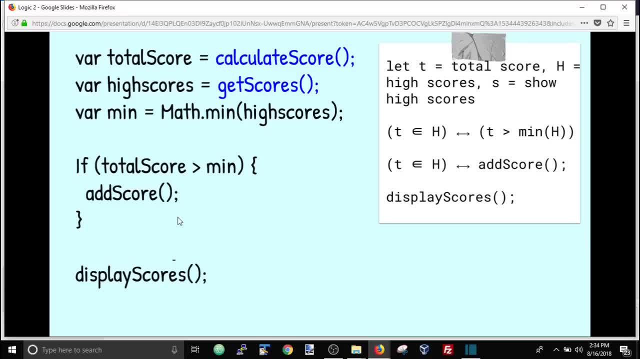 function to find the minimum value in the set. if total score is higher than the minimum, we're going to execute the code to add that total score to our high score list and no matter what, In any case, we're going to go ahead and we're going to display the high score list for the player to see. 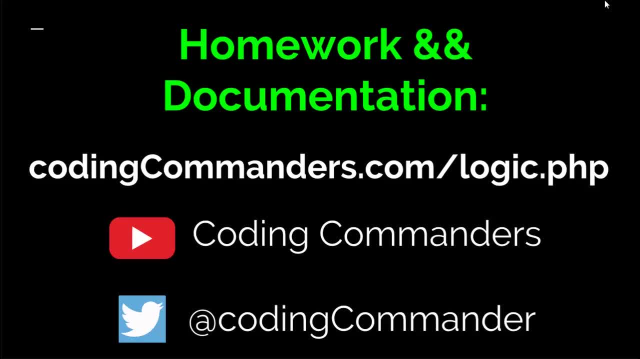 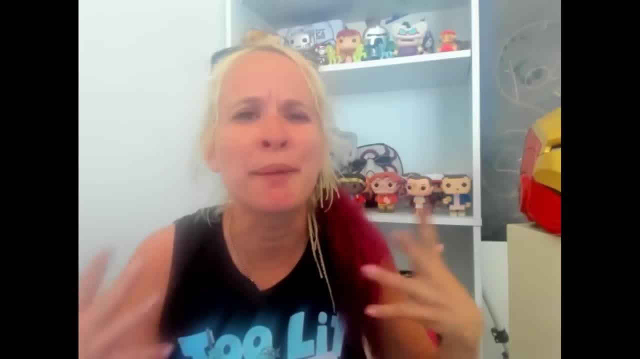 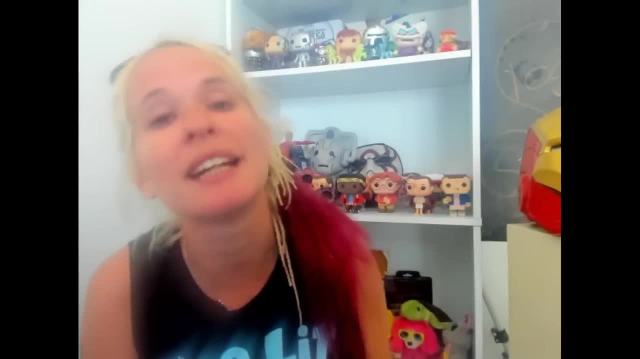 Thank you for watching my video. Don't forget to go to codingcommanderscom. slash logic dot php. with logic programming, math. The only way you get better is by practice. You watch the video, you learn the concept, then you have to apply it. 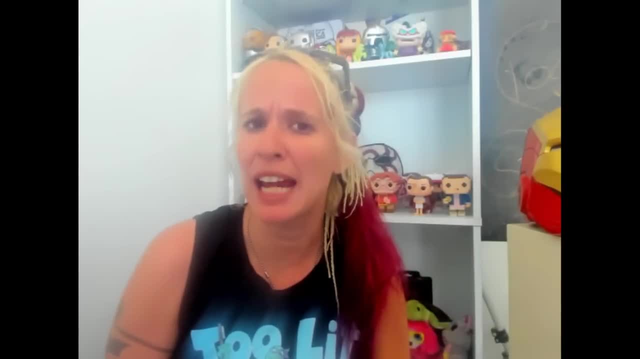 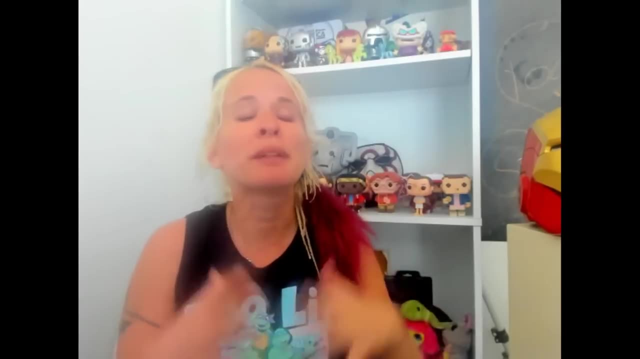 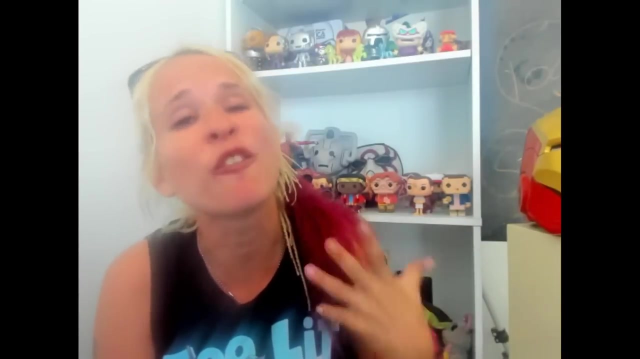 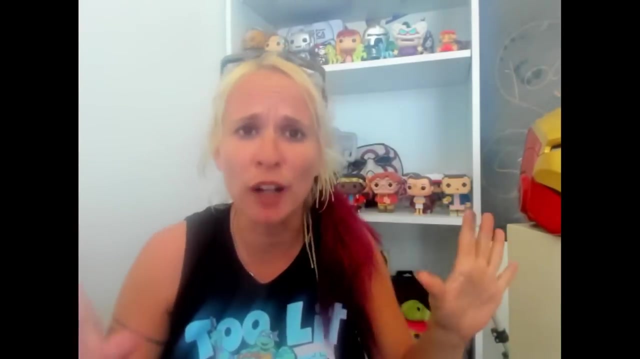 So please check out the homework. The last video I had a little quiz for homework. This time I have three word problems. If you have any questions, please feel free to comment on this video. I will be checking the comments. If you complete the homework and you feel like you want me to look it over, you can go ahead, upload it to GitLab, GitHub, wherever you want. 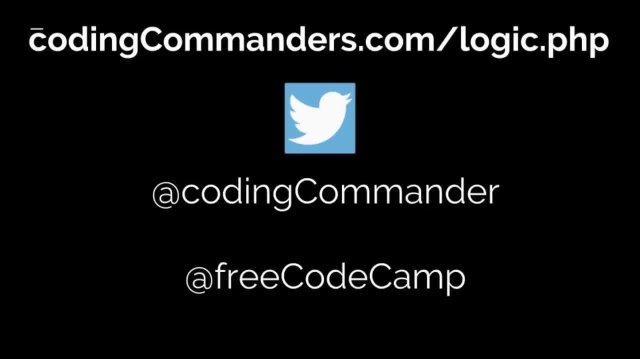 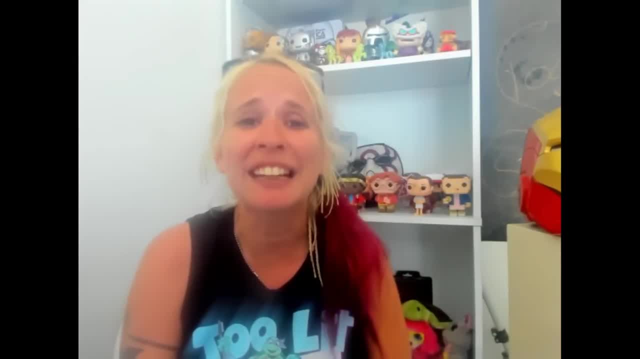 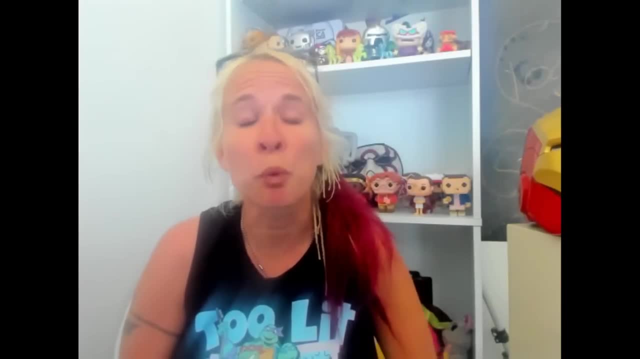 Tweet the link. Make sure to mention me in free code camp. I will try to get to everything Everybody. if you do reach out- and it's been like a couple of days you haven't heard from me- feel free to give me a little nudge in the next video of the intro to logic for computer programmer. free code camp series. 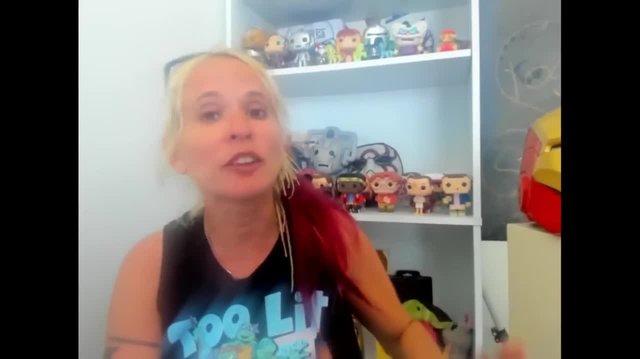 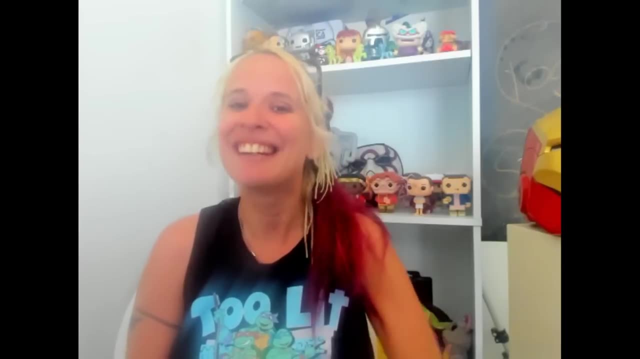 I am going to apply all the set theory we learned today to some actual sequel. We're going to learn how to make awesome databases using set theory. Thank you again for watching my video and until next time, Happy coding.